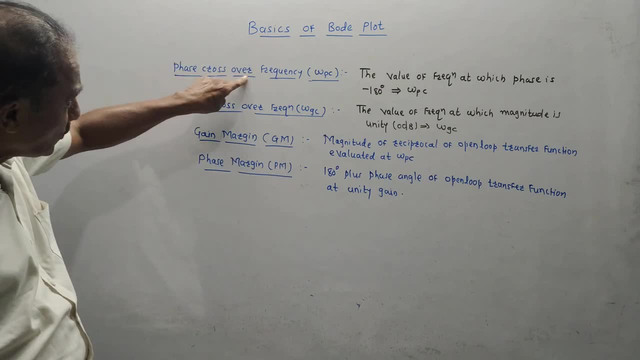 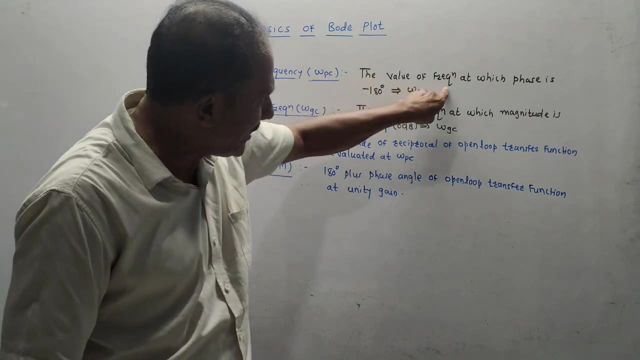 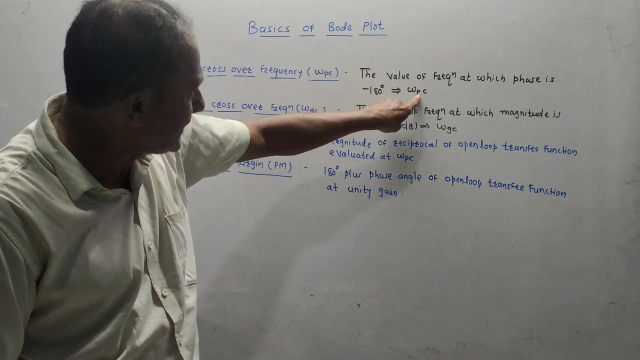 will discuss few important definitions. First is phase cross over frequency. It is denoted by omega PC. PC stands for phase cross over The value of frequency at which phase is minus 180 degree. That is called phase cross over frequency. Next is gain cross over frequency. 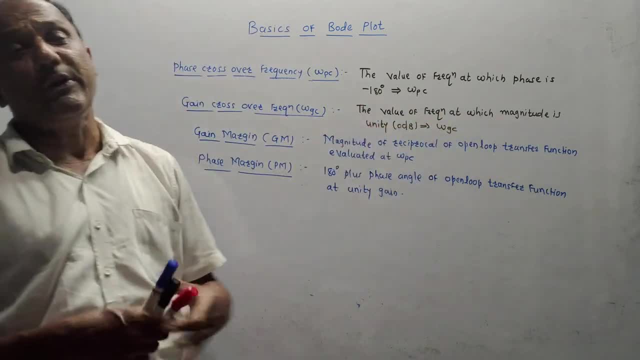 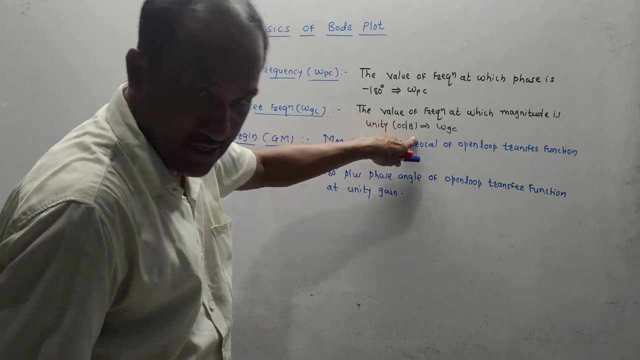 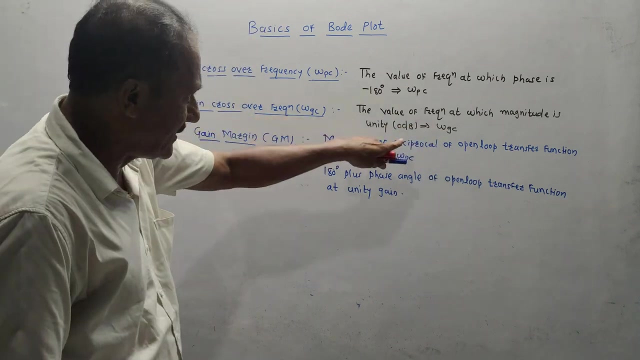 This is the value of frequency at which magnitude is unity. Now we have to use dB scale, decibel scale. Unity magnitude means 0 dB. I will explain this while drawing And the actual graph. This is corresponding to gain: cross over frequency. That means the. 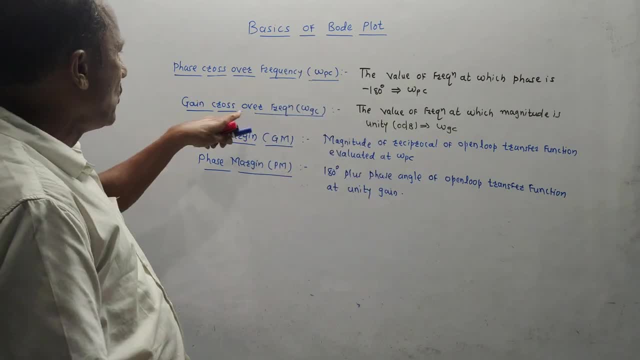 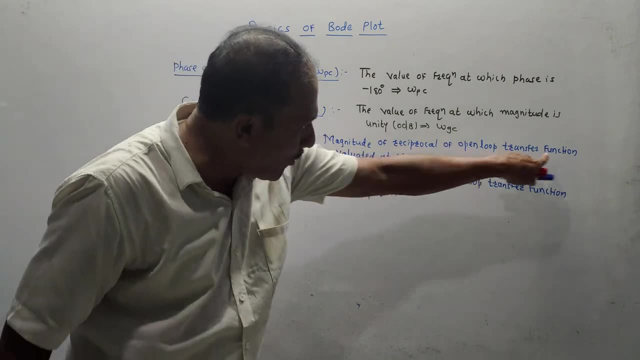 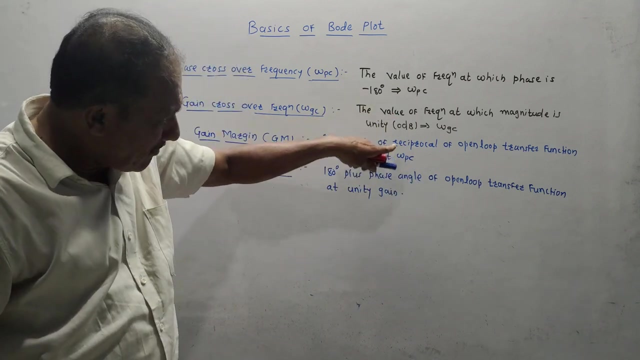 frequency at which 0 dB reading comes. that is related to omega GC. Next is gain margin, that is GM Magnitude of reciprocal, of open loop transfer function related at omega PC. Now this will not be clear here On the graph paper. I will explain to you what is the actual. 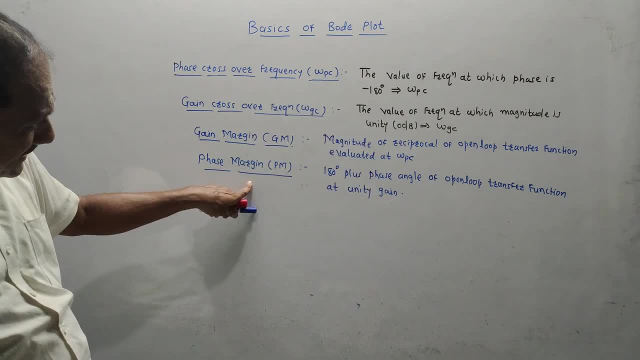 meaning and how to measure the gain margin. Now, this is the actual graph. This is the actual gain margin. Next is phase margin. It is 180 degree plus phase angle of open loop transfer function at unity gain. Now to draw the diagram, you need to know certain basic 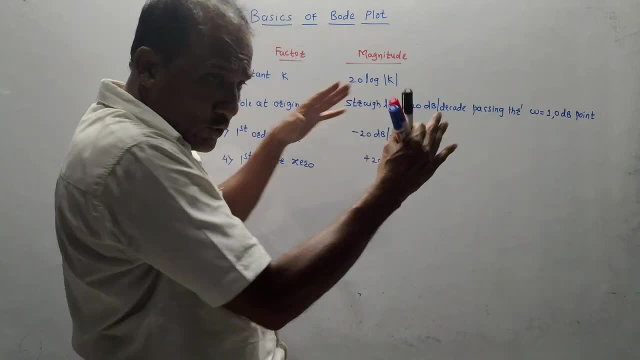 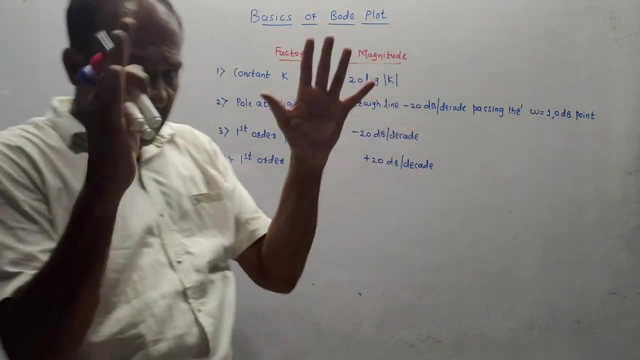 rules. Now see, there are many rules. If I want to write all the things in the tabular form, then there will be another column of phase and there may be many parameters, But I have compressed the things. You just have to remember four things. Rest of the things. 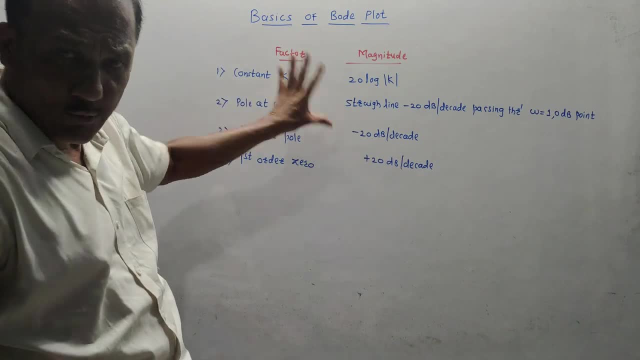 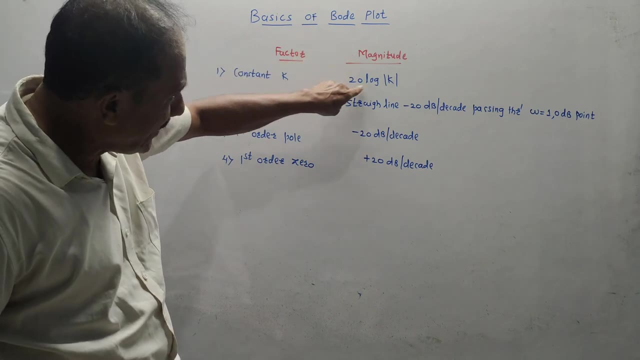 I will explain while explaining the numericals. So just remember this formula. First, constant K. That means there is a constant factor in the equation. So its magnitude will be 20 log mod of K. K is the value of constant Value of phase. I am not purposely writing. 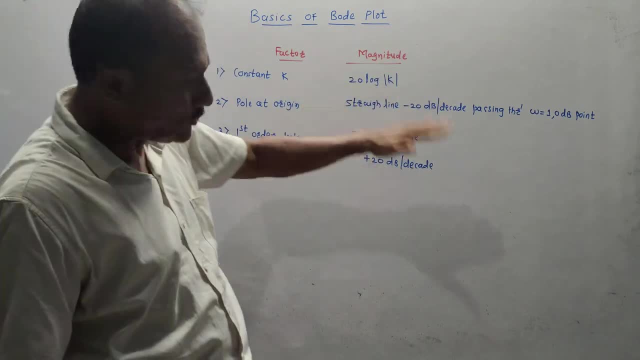 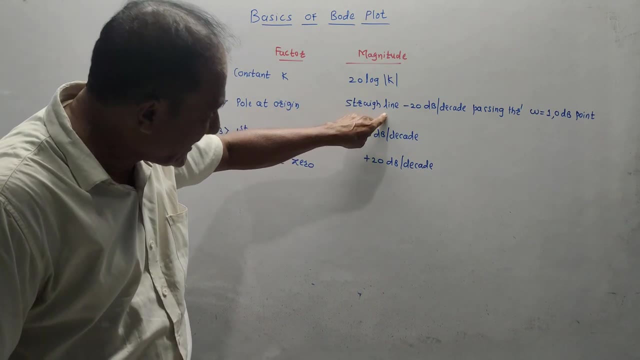 it. I will explain you how to do it, how to manage the phase while solving the numericals. Alright, Second, pole at origin. That means there is a pole at origin that will be corresponding to straight line of minus 20 dB per decade. So this is the value of the pole at origin. So I have written a straight line of minus 20 dB per decade. This is the value of the pole at origin. So I have written a straight line of minus 20 dB per decade. This is the value of the pole at origin. So I have written a straight line of minus 20 dB per decade. 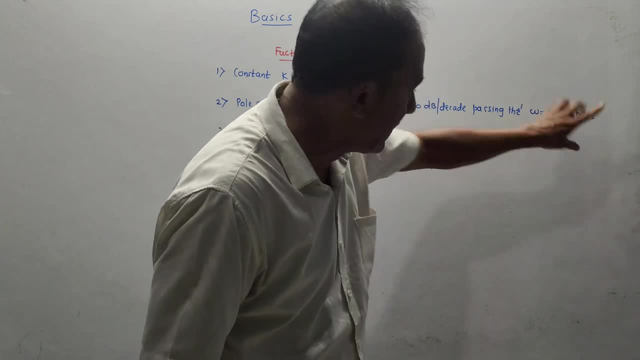 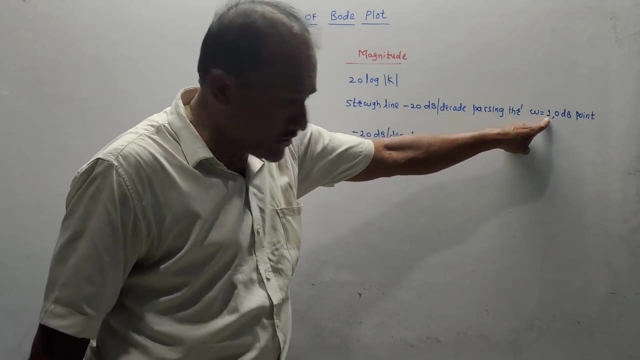 As a rule, the number of poles at origin possibility is zero. So you assume that what will be the magnitude of the pole at origin? For that, only the line of pole at origin is a function of the 2 currencies R into K. I am done. 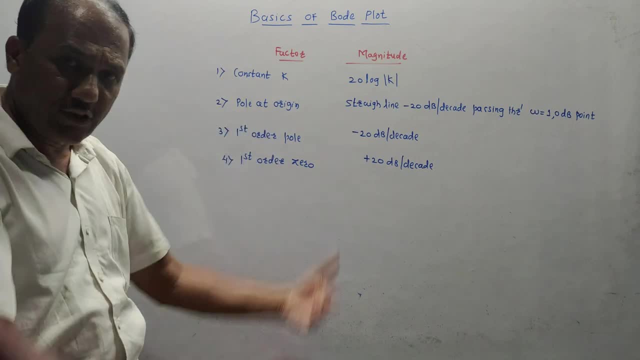 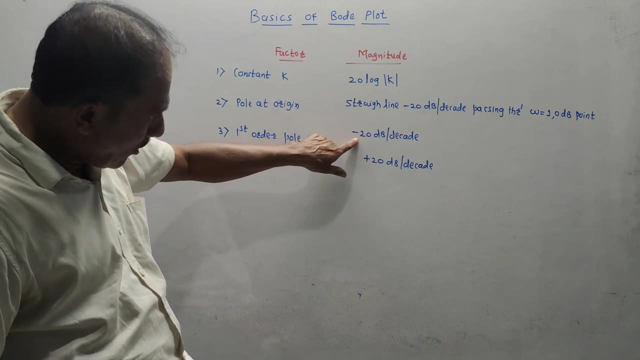 So let me explain. what is the magnitude of the pole at origin? If there is a Porsche angle line for the pole at origin, then the energy that comes from the point where the pole is formed. So that is the measure. Okay, So let me explain. 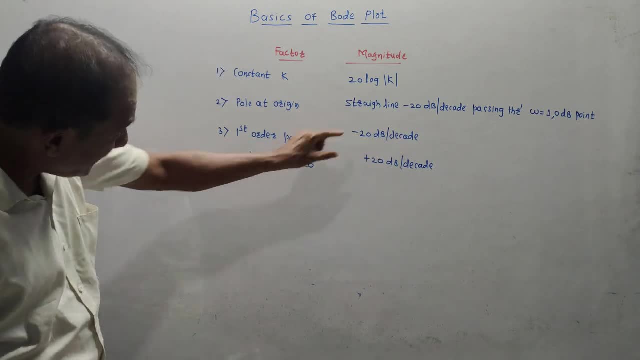 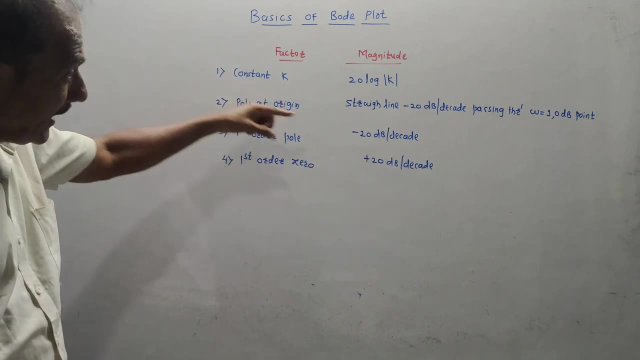 Now you would understand again. I am melt them all together now It will create into 20 DB per decade. first order: 0 is the exact opposite: pole kele minus 20, 0 kele plus 20 DB per decade ab. second order: pole hai to iska double karna hai minus 40 DB per decade. 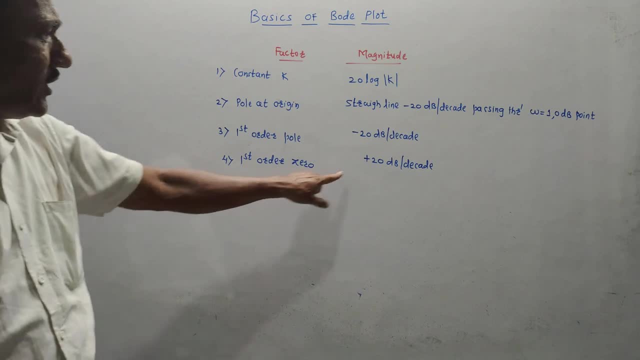 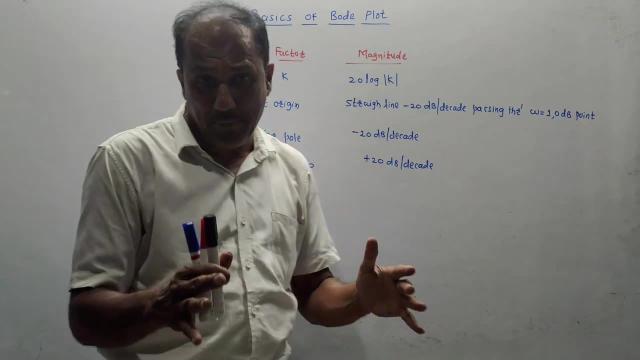 third order pole hai to minus 60 and so on. likewise, second order 0 hai to ye first order ka plus 20 hai. second order ka plus 40 DB per decade. hoga ab actual graph paper pe ye kaise implement karna means scale, kaise choose karna hai how to identify different frequencies. 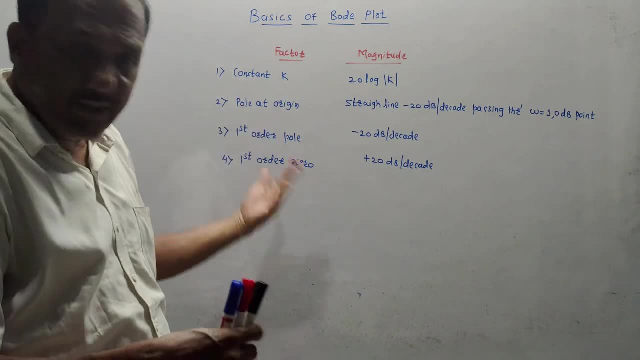 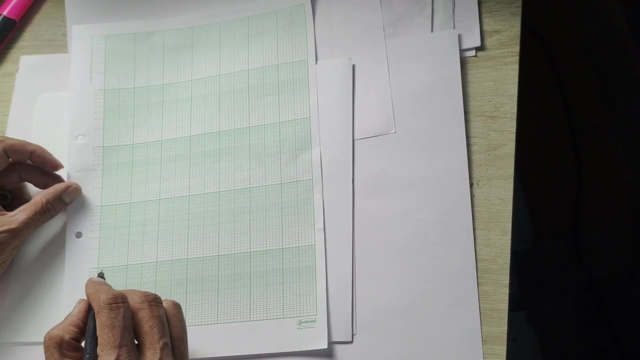 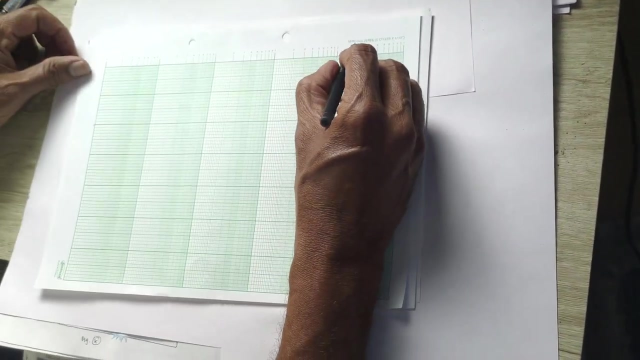 how to mark different points. ye sab mai aapko actual graph paper pe explain karta ho. so let us move to the semi-lock paper. Dear students, this is the semi-lock paper, lekin ye aapko aise pakarna hai, jaha pe yaapko dikhai dega semi-lock paper five cycles, and so on. so 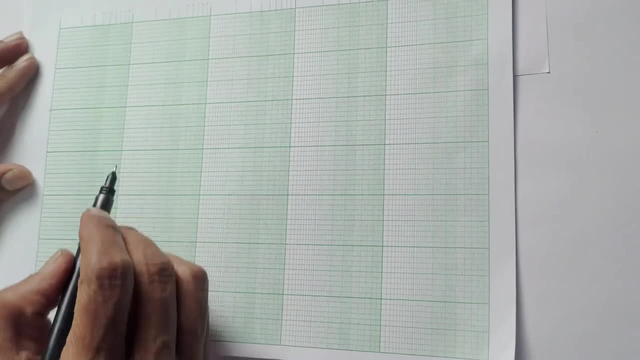 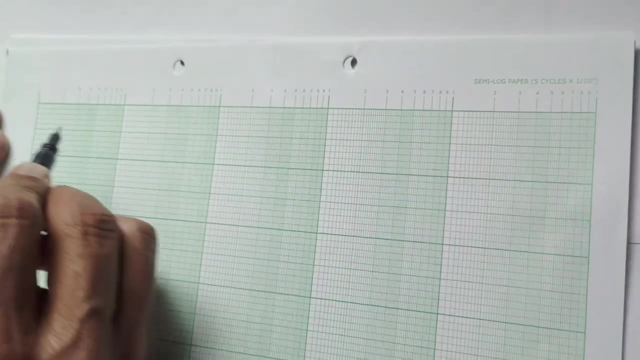 this is the semi-lock paper. you will have to hold it like this: ab dekho, this is the semi-lock paper. so ye jo axes hai, this axis logarithmic scale. Observe it carefully. The first value is 1.. Again, this value is 1.. 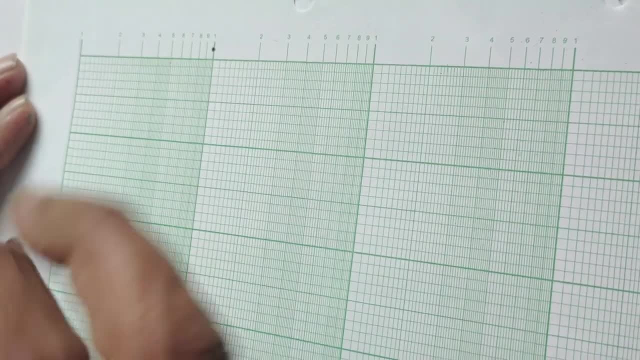 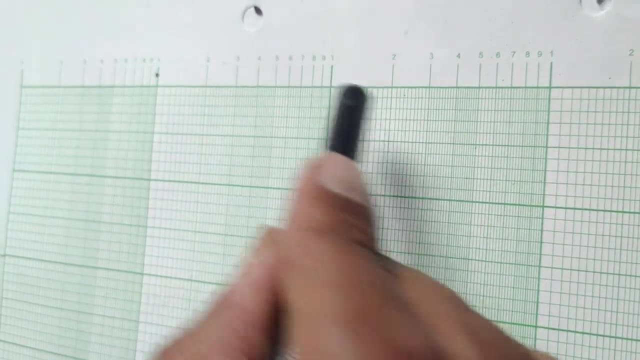 In between. the readings are 1,, 2,, 3,, 4,, 5,, 6,, 7,, 8,, 9.. But these are uneven readings, unequal. Look again. Here again, there is a slot where 1 has come again Again there. 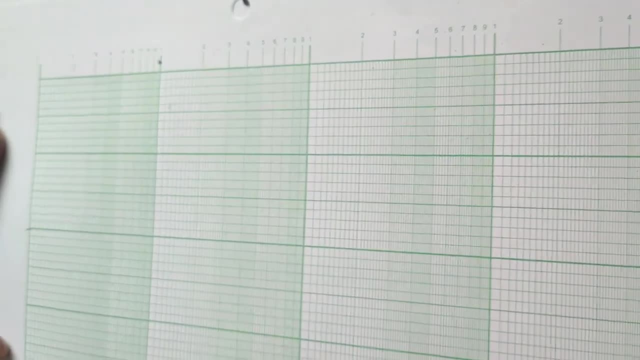 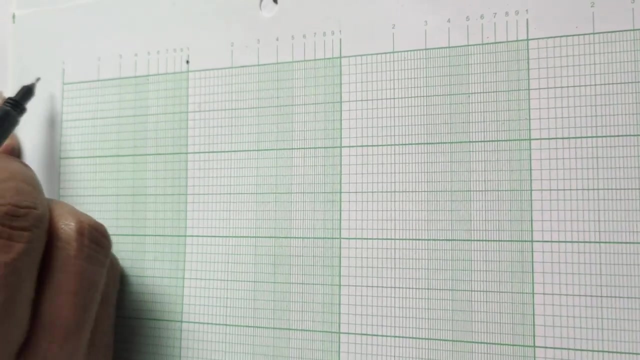 is one slot, Again 1 is marked, and so on. Likewise there are 1,, 2,, 3,, 4, 5. 5 slots. Now how to take the reading. Let us say for first line, where 1 is written. I will: 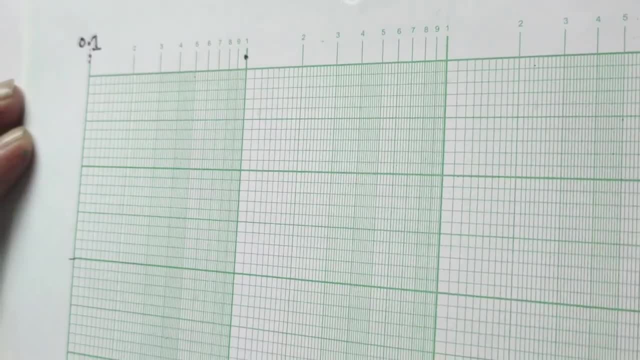 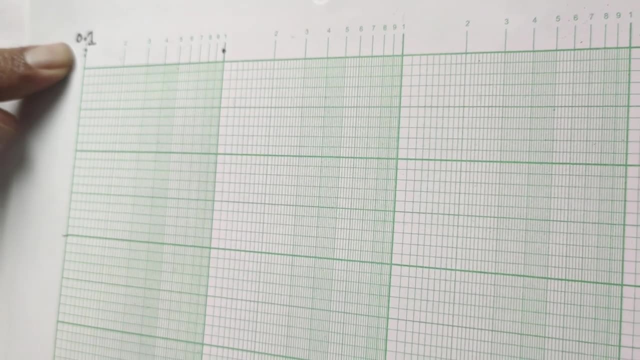 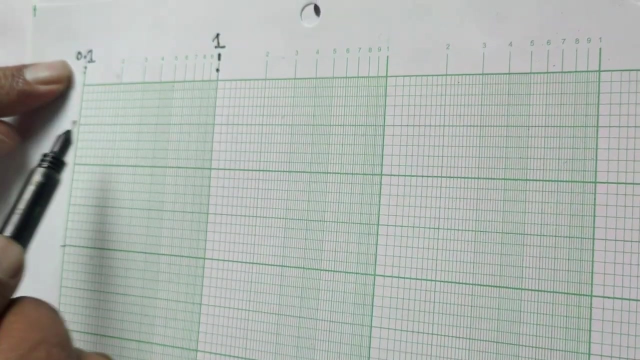 say this point is 0.1.. It is not necessary to assume this reading, But it will make the calculation simple Here. I have assumed that this is the reading of 0.1.. Next one, where it is 1, I will say this reading is 1.. Now, how to prepare this. Look the first reading. 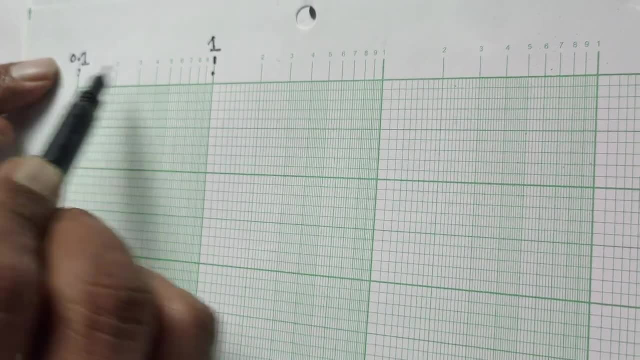 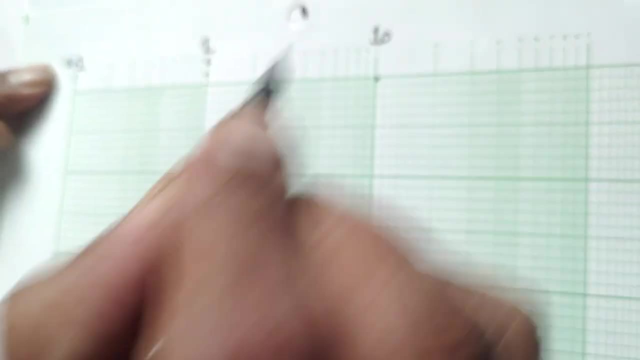 point is there. In between there are 10 lines, So 0.1 into 10.. This reading is 1.. Next one, where this one. Here I will write 10.. This reading is 10.. Likewise next reading. 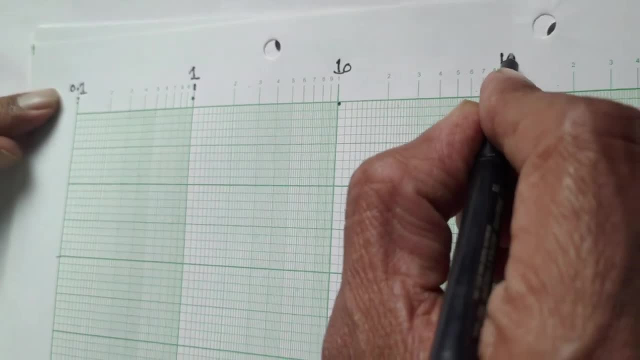 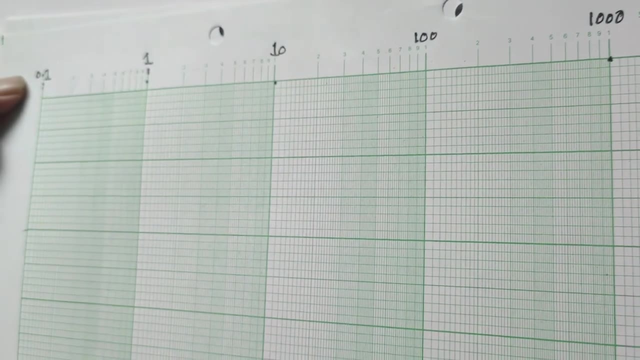 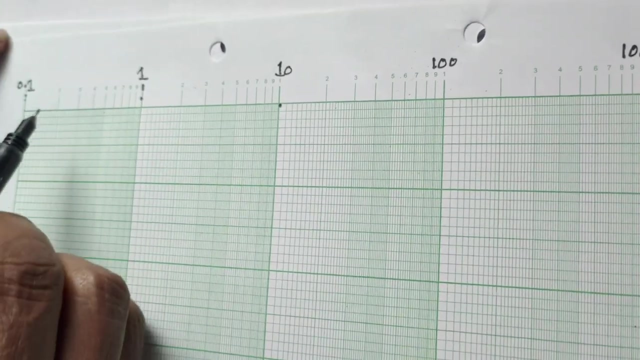 will come on this line where 1 is written, Here, reading will be 100.. Next line, where 1 is written, reading will be 1000, and so on. Now how to mark the values, Actually, these readings which I have written: 0.1,, 1, 10, 100, 1000.. These are the readings corresponding. 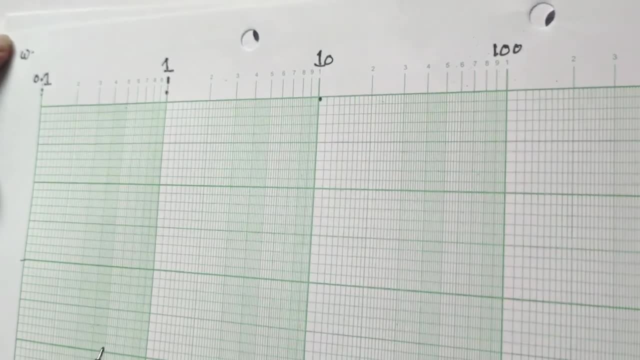 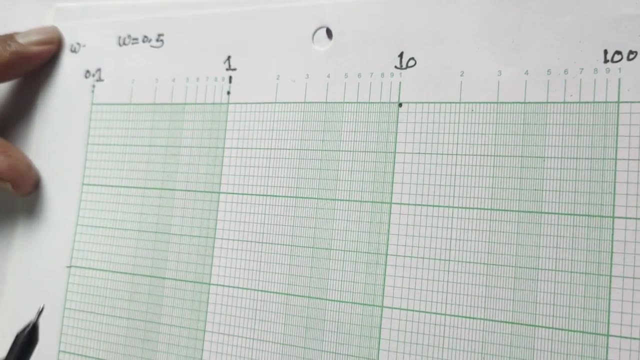 to omega. Omega is the frequency. Suppose. I have to mark this reading as omega equals to 0.5.. So how to mark this reading as omega equals to 0.5? Look, here it is 0.1 and here it is 1.. So where should I see 5?? 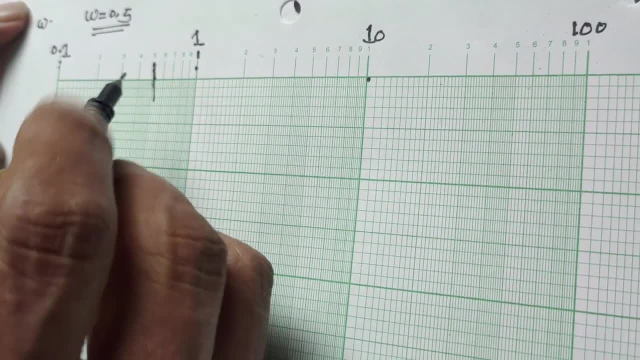 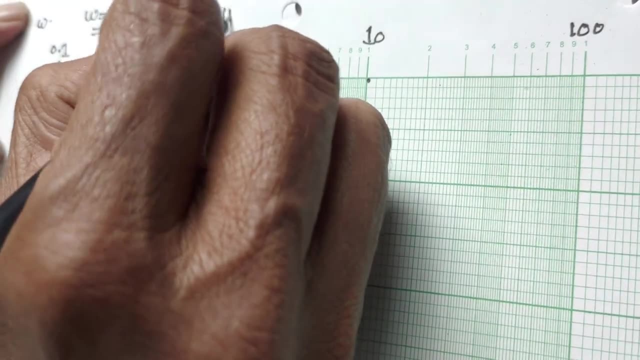 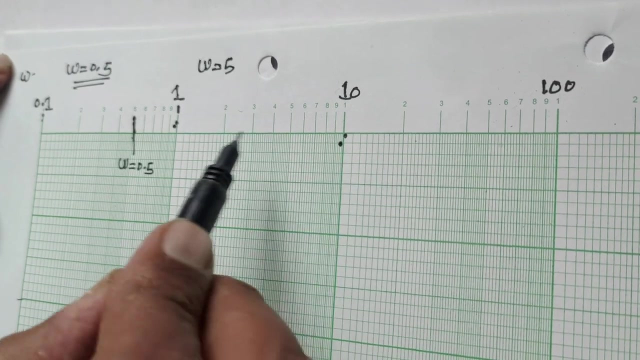 This line is of 5.. So this line corresponds to value of omega equals to 0.5.. Next reading, suppose I want reading of omega equals to 5.. Now look here: omega equals to 0.5 and here it is 1 and here it is 10.. LOCAL READING OF 5. So this can be written as 0.5. So 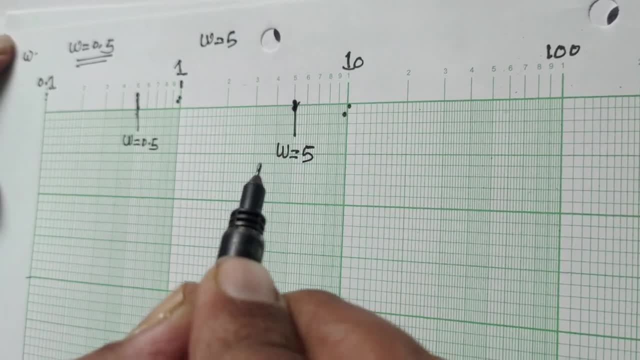 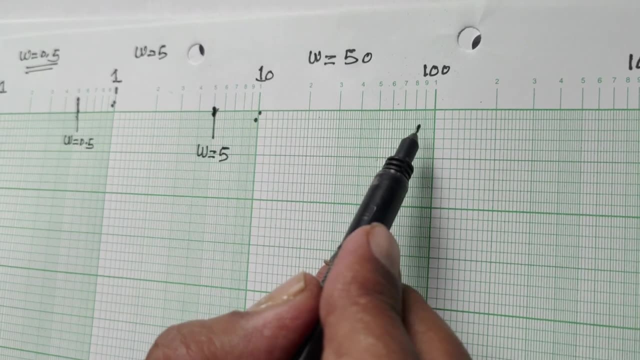 this is one. So this line corresponds to omega equals to 5. So let me marklerin Omega equals to 50. Omega equals to 5 is the scale of 10.. Now I want to mark reading for omega equals to 50. Next Wnt to mark 50.. So this can. 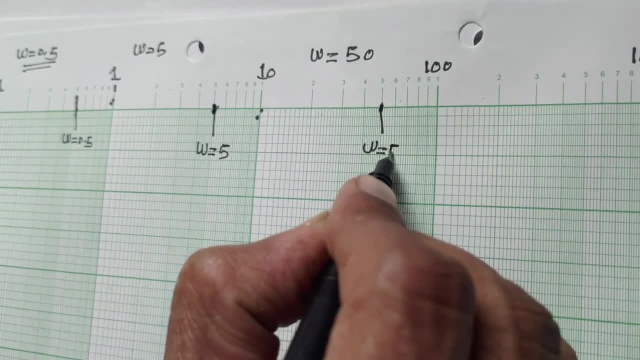 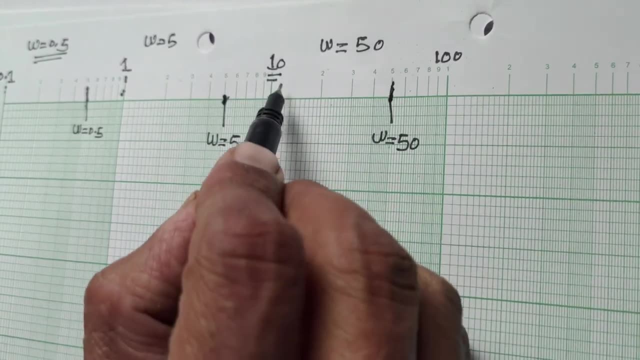 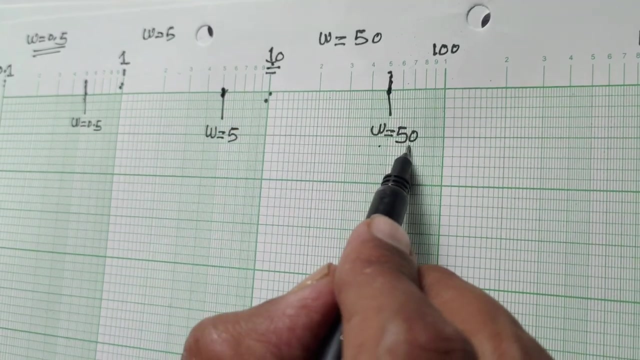 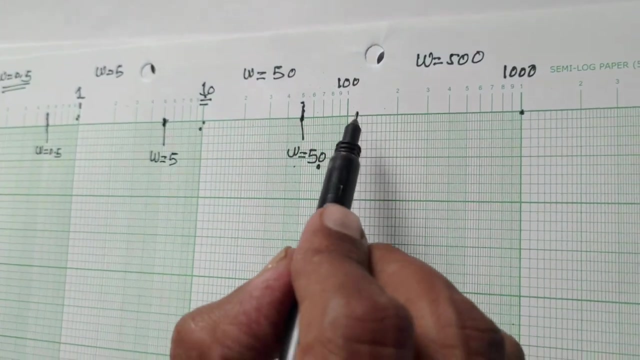 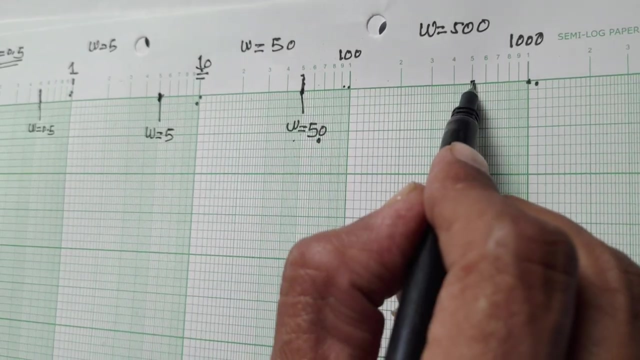 be written as one Radical reading equals to 10 and this is a integral. This is interesting. So this is thekhari line, block Here: 2, 4.. then this reading is of 5, in between 10 and 100, this reading is for 5, so just multiply it 5 into 10, it will be corresponding to 50,. now let us say I want to mark reading for omega equals to 500, so it will be between 100 and 1000,. again, check for the line of 5, this is the line of 5, so 100 into 5 will be 500, so this reading will be corresponding to omega equals to 500,. 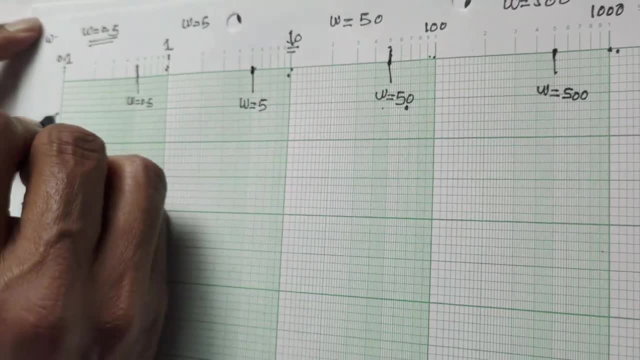 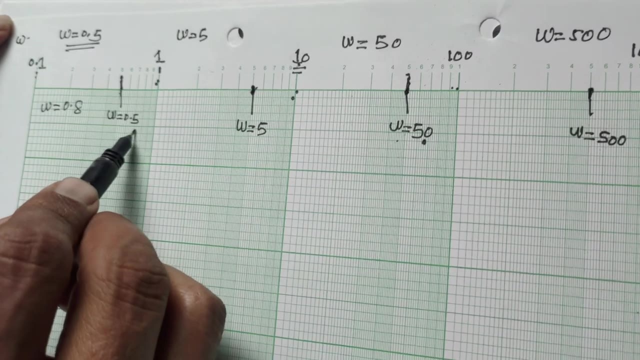 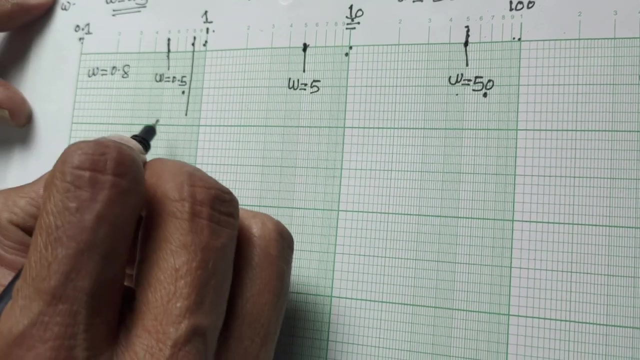 likewise, you can mark any reading. let us say, I want to mark omega equals to 0.8,. how to mark this reading? very simple: like we have marked 0.5, in between 0.1 and 1, where do you want to see the line of 8, this is the line corresponding to 8, so this reading will be corresponding to omega equals to 0.8,. 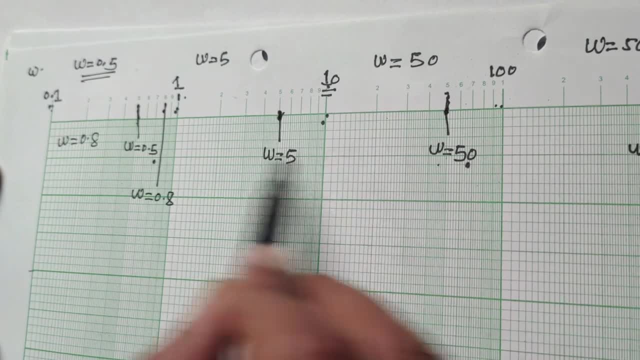 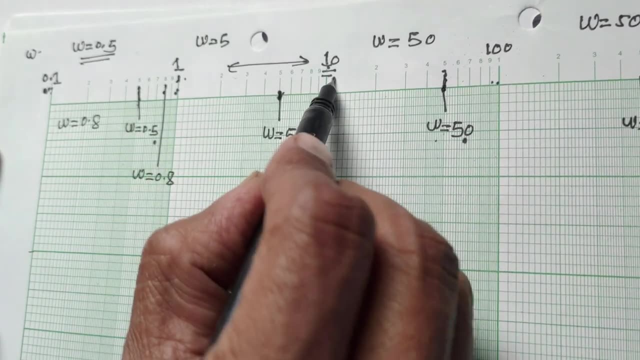 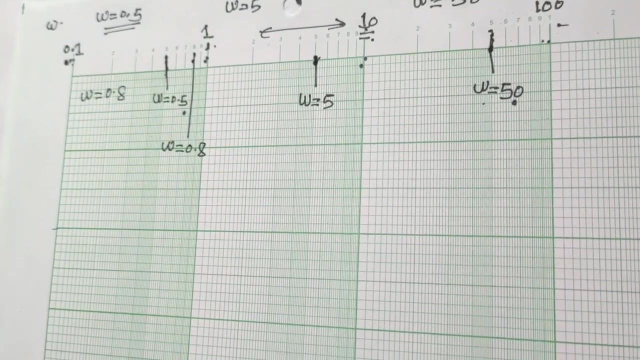 likewise, you can mark any reading on the x axis. these are the readings of x axis. so I have started from 0.1,, then 0.1,, then 1,, 10,, 100,, 1000 and so on vertical line. here we have to take normal readings. now I will explain the next part along with this. 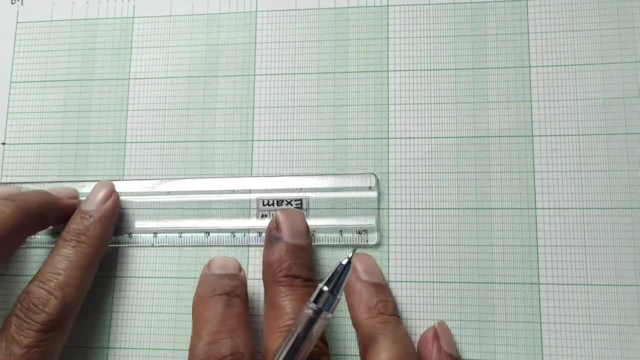 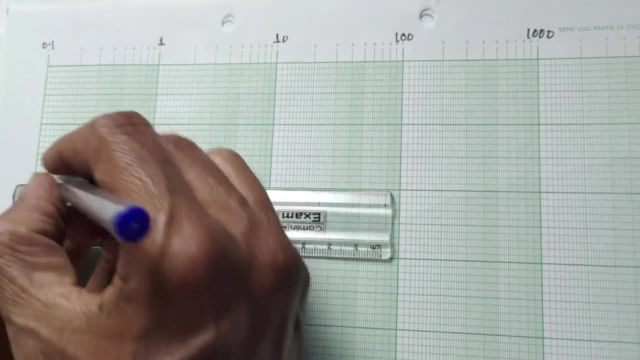 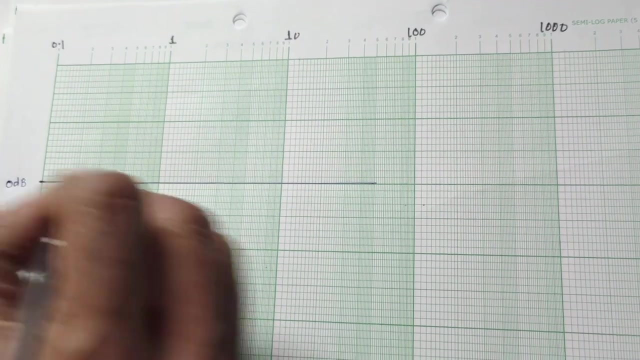 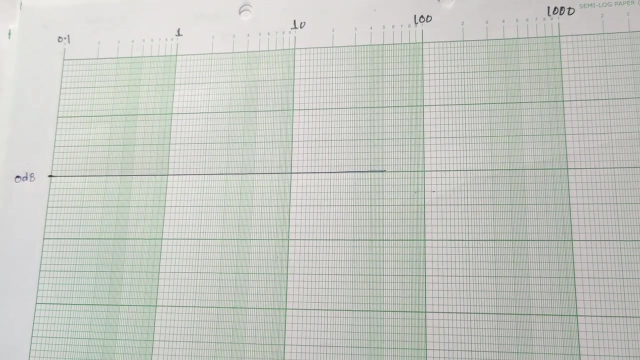 now, see, suppose I want to mark magnitude plot, so somewhere I will have to consider a reference line. remember, for magnitude the reference line is 0 dB line. that is 0 dB line. this is the reference line. now, see, as I have told earlier, you need to draw two graphs on the same graph paper. 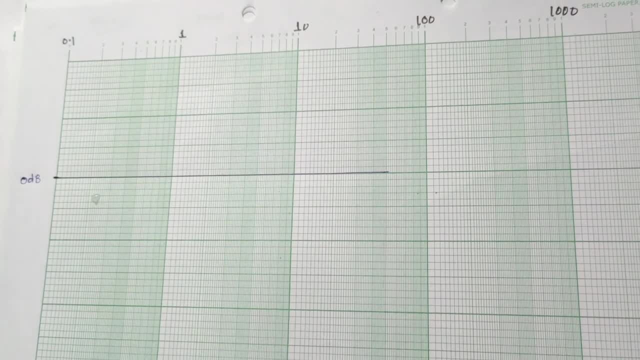 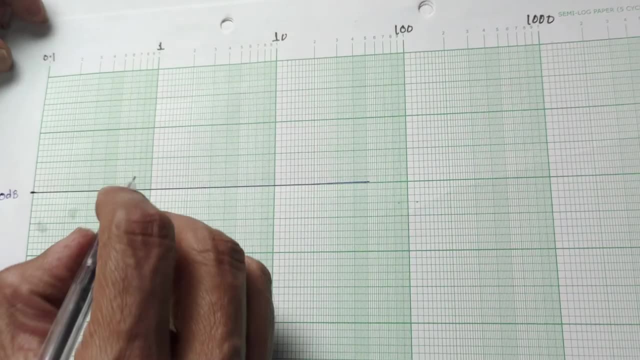 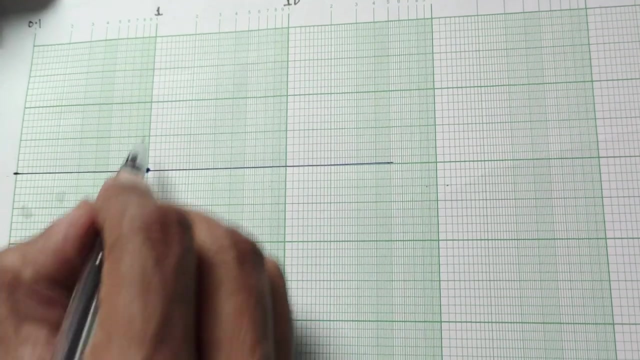 one is magnitude plot and the other is unit to draw phase plot. now for magnitude plot, I have taken 0 dB reference. now I have to draw more reference lines like: see this is 1 line and this is 0 dB line. this is point of intersection for 0 dB and frequency corresponding to 1,. 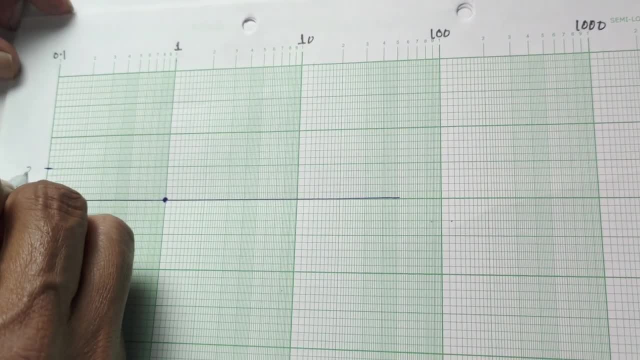 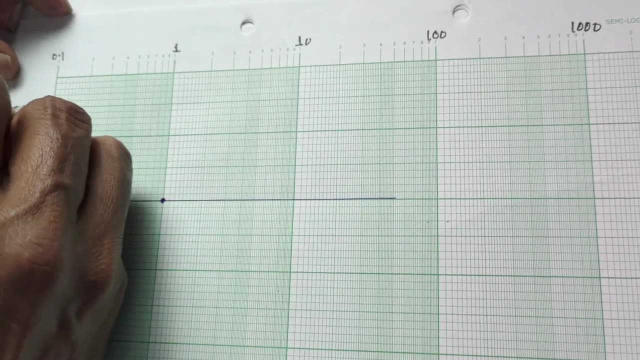 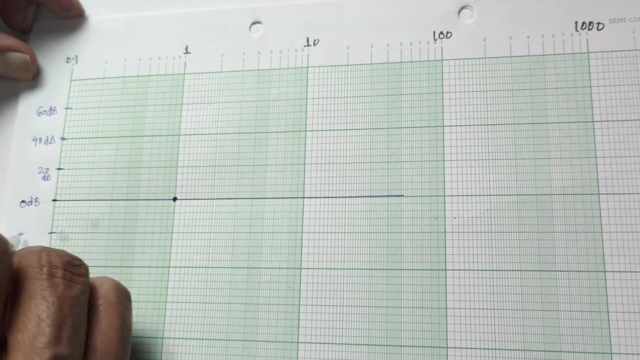 now I will mark some scales here. suppose this is 20 dB, this is 40 dB, 40 dB, this is 60 dB, this is the reading above 0 dB, so I have considered it positive. below that will be minus 20 dB, below that will be minus 40 dB, and so on. 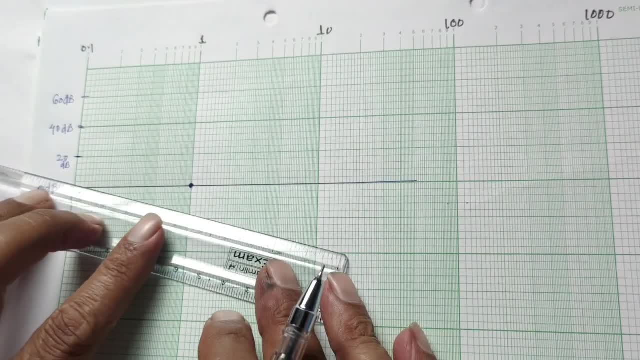 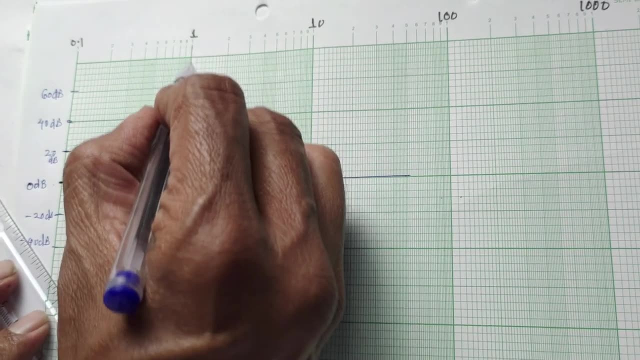 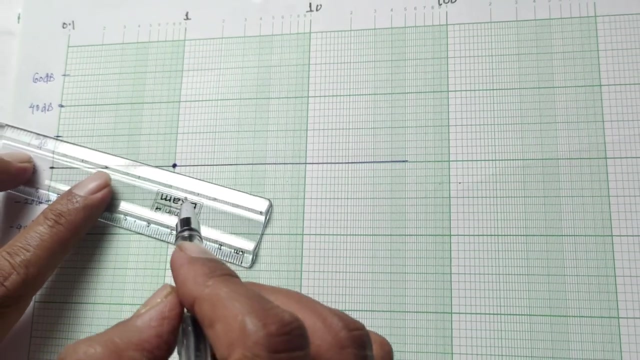 now if I will draw one line from 20 dB to this point. and which point is this? remember this line of 0 dB and line of 1, where intersection comes. this is the point here where I have marked plus 20 dB from there to here. if I draw one line like this: 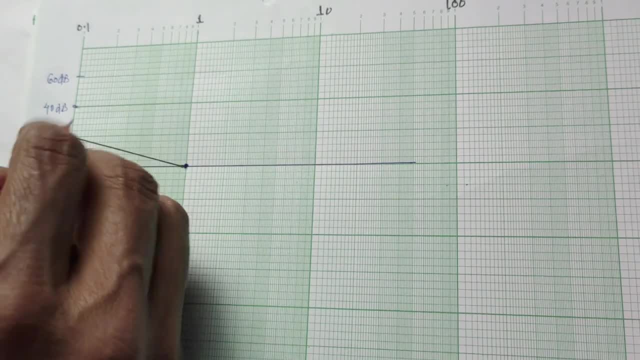 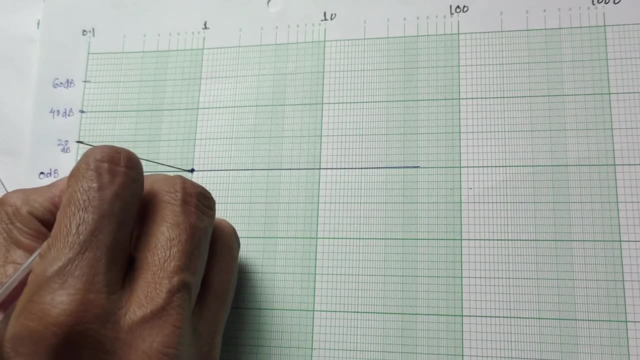 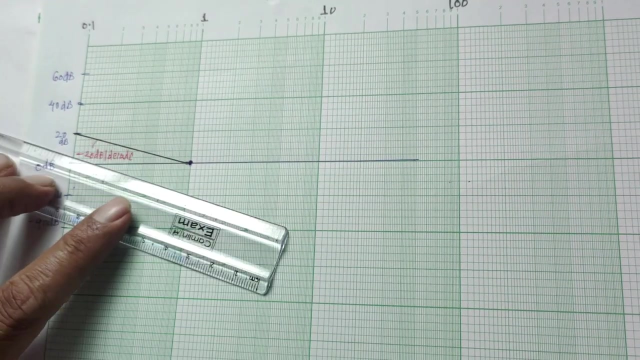 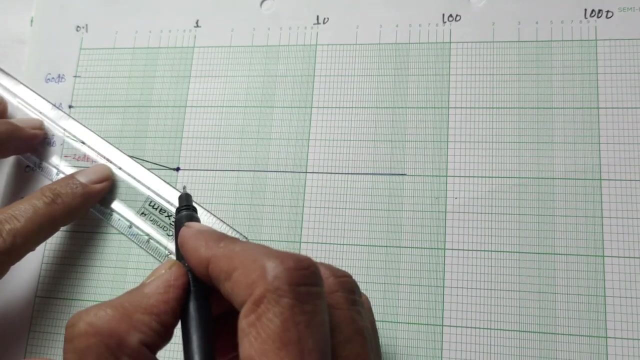 its slope will be. this slope of this line will be minus 20 dB per decade. why minus 20, because this line is decreasing, so its slope is negative. it is minus 20 dB per decade. now this is point of 40 dB. see, this is point of plus 40 dB. from here to reference point, if I will draw one line, 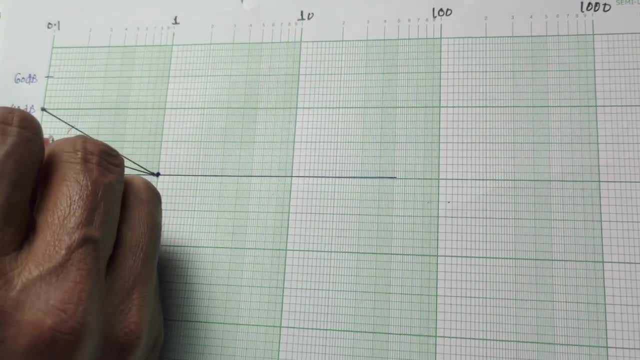 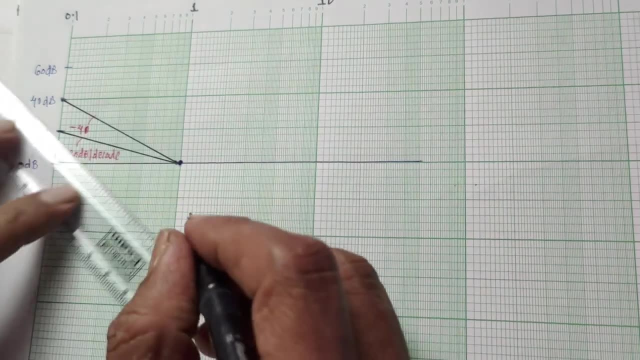 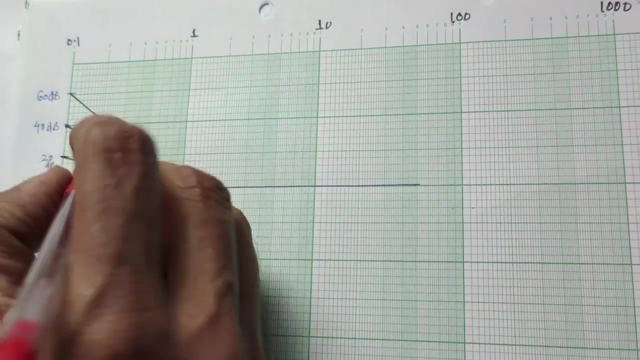 then slope corresponding to this line will be minus 40 dB per decade. I am not writing dB per decade by default, it is dB per decade. likewise, from 60 to this point I will draw one line again. this is a reference line. this slope will be minus 60 dB per decade. 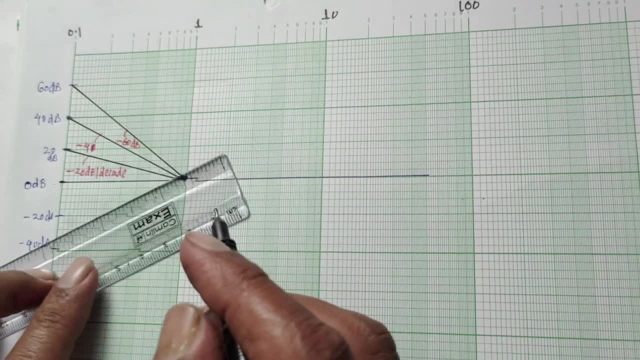 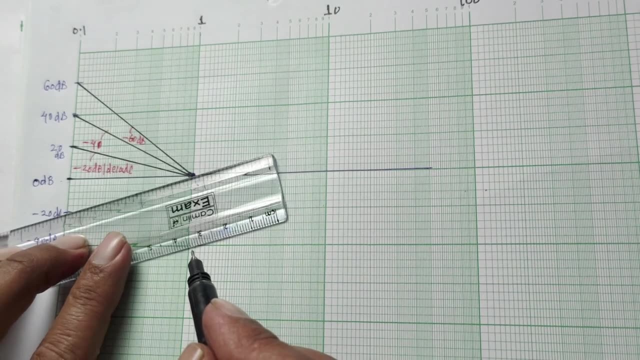 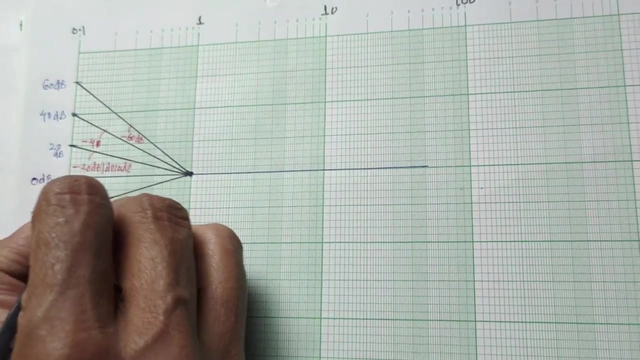 now, as you can see, this is a line of minus slope. if you want plus slope, it is very simple. it is the exact opposite. this is a line of minus 20 dB from here to reference point. if I will draw one line, this one, its slope will be plus 20 dB per decade. simple tricks. 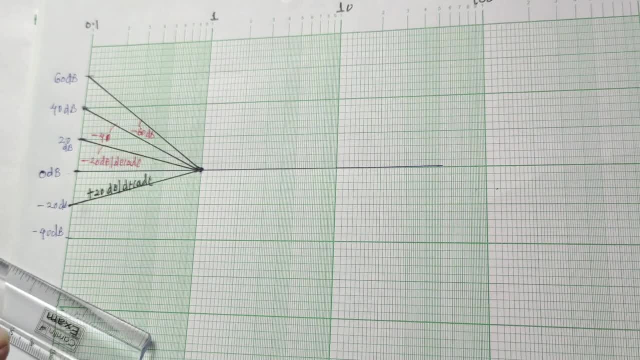 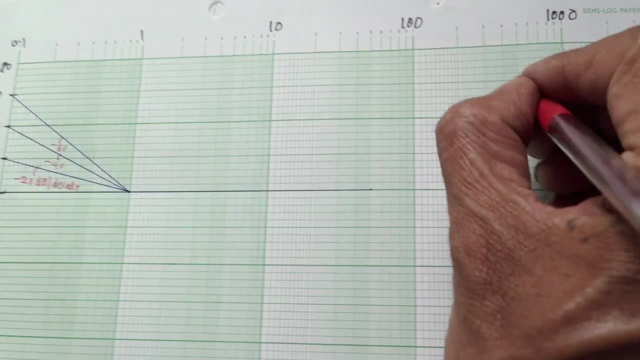 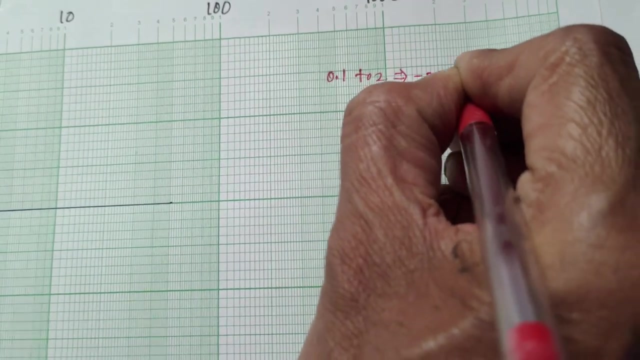 keep this in mind. if it is an increasing line, then its slope will be plus. if it is a decreasing line, then its slope will be minus. suppose I have to mark some readings like from point one to two. I need to draw a line of slope minus 20 dB per decade. 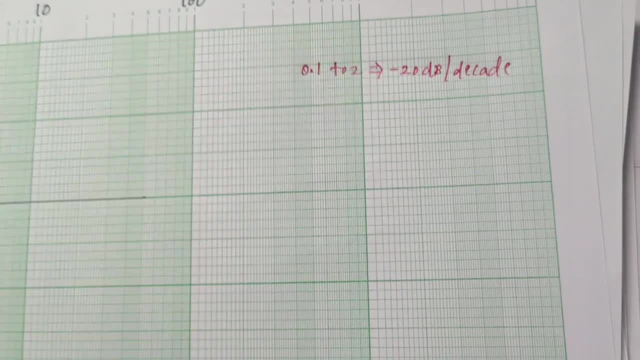 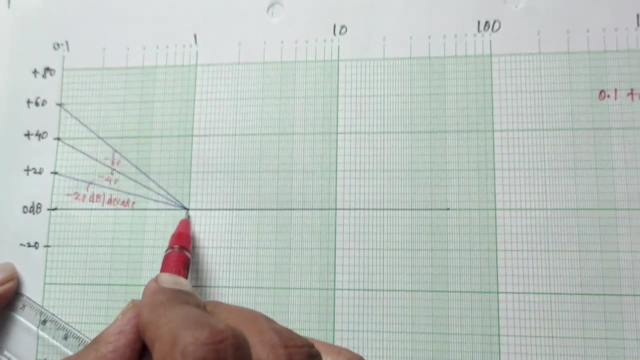 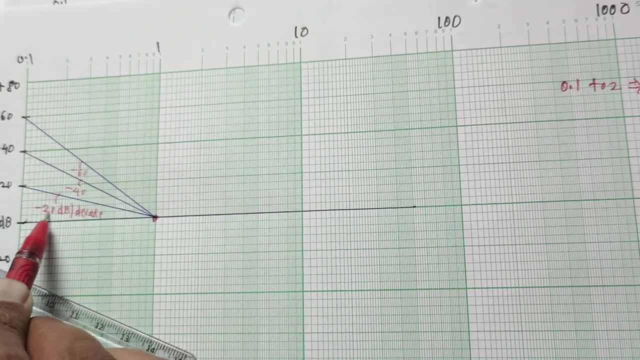 how is this drawing? Now see this reference line. we have already drawn this line like: see, this is a reference line of 0 dB. the slope of this line is minus 20 db per decade. now what is my requirement? i want to mark the line. 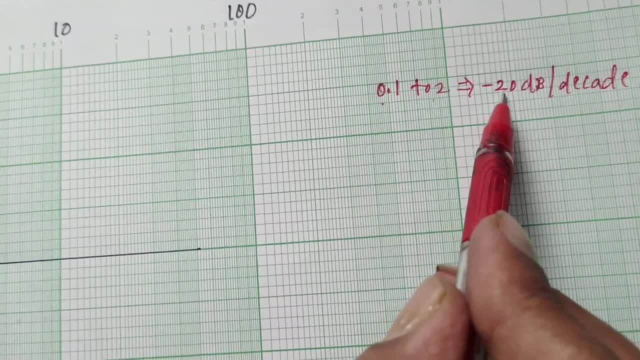 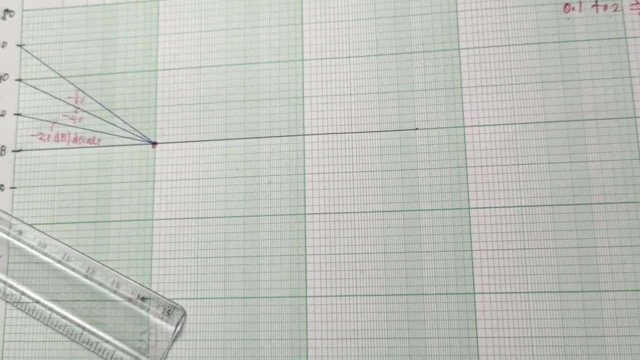 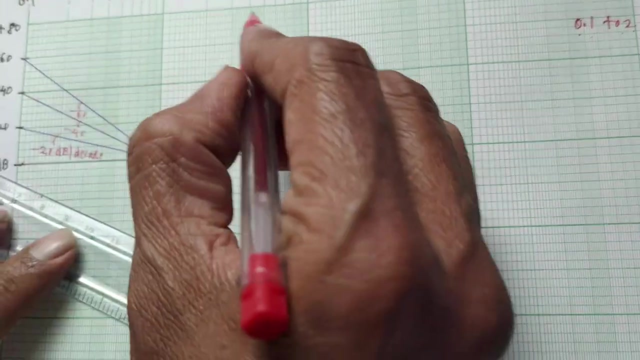 from 0.1 to 2, whose slope should be minus 20 db per decade. now how to draw this line from minus 20 db to 0.1 to 2 means this is the point of 0.1. this is the point of 0.2. 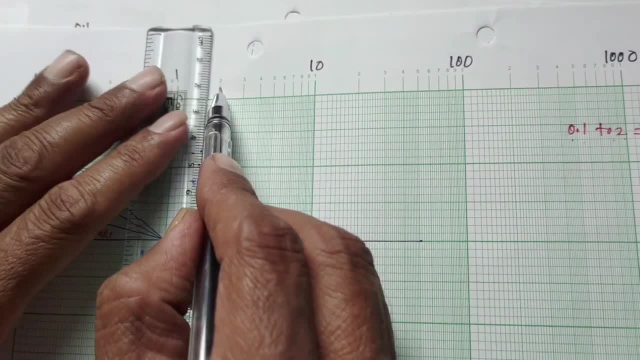 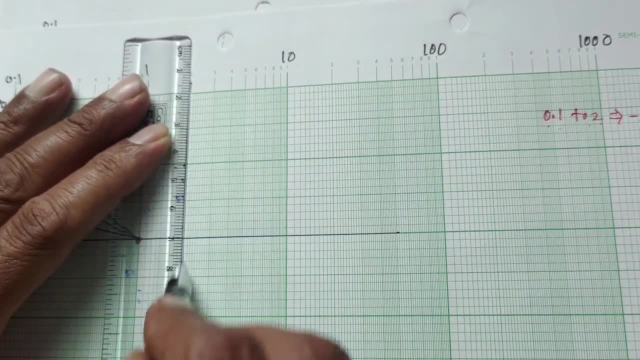 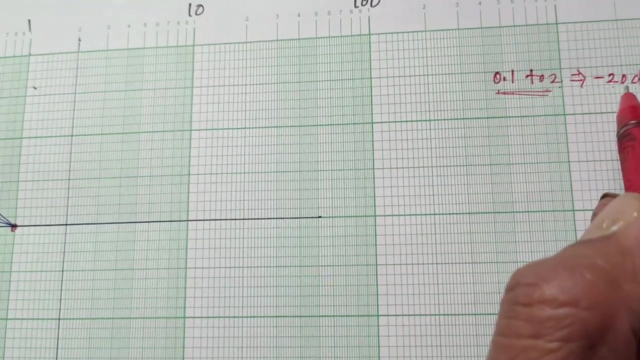 first mark the point of 0.2 for reference. this is the point corresponding to 0.2, see between 1 to 10. this will be the reading of 0.2. first i will mark a reference line related to this. what is my requirement? 0.1 to 2. i have to draw a line of minus 20 db per decade. 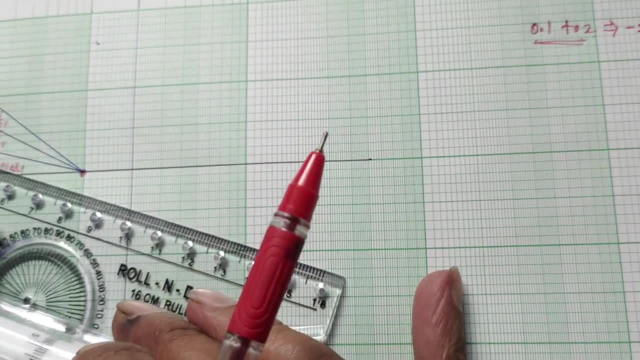 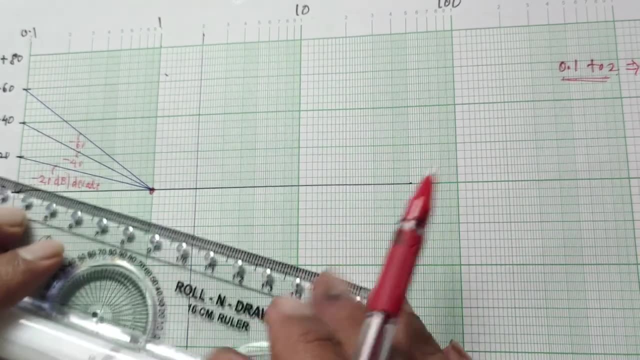 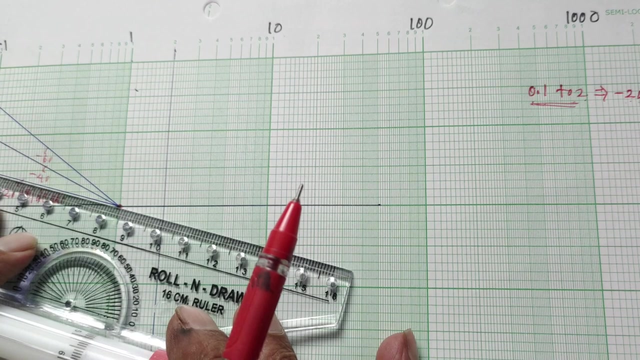 now how to draw this line. already i have drawn a reference line of minus 20 db per decade. i am talking about this line. i have drawn this line till one reading. i have to just extend it till 0.2. so this has to be parallel means i have to extend it further. 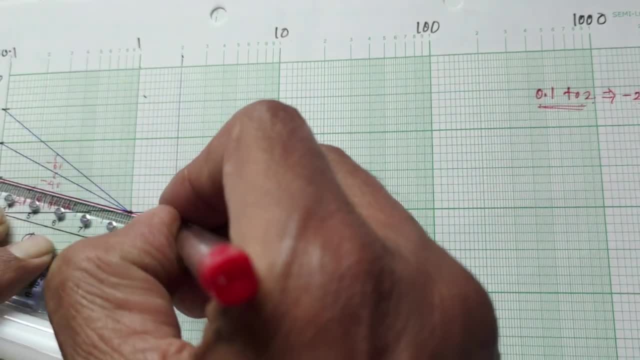 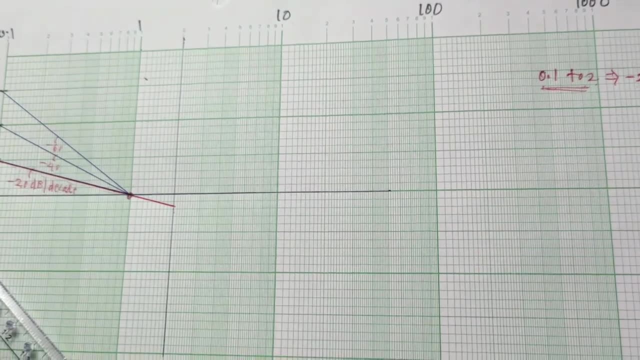 so this line will be from 0.1 to 2, whose slope is minus 20 db per decade. so this line will be from 0.1 to 2, whose slope is minus 20 db per decade. now, this will be from 0.1 to 2, whose slope is minus 20 db per decade. 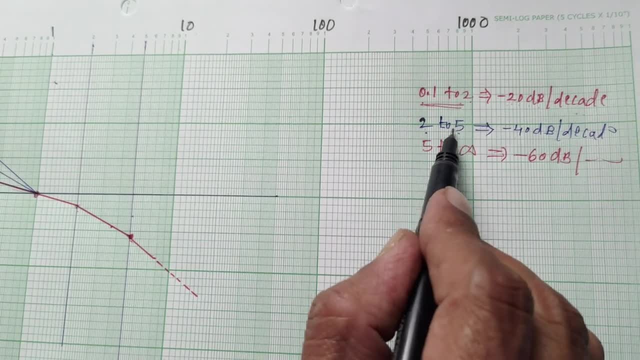 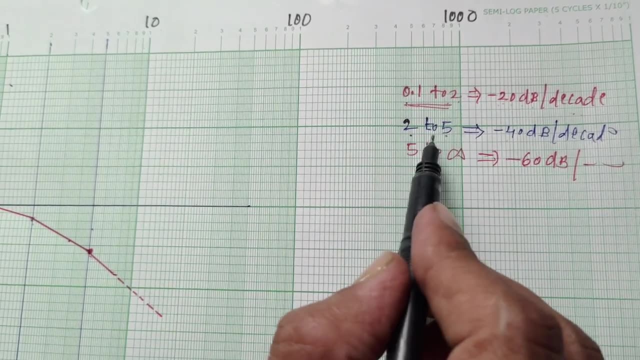 now we have to mark some readings. and if we have to mark some more readings, suppose we have to draw this line of minus 40 db per decade till 2.5. i have written this already, just to save the time now. as you see, a reference line of 2 means this is the reading between: 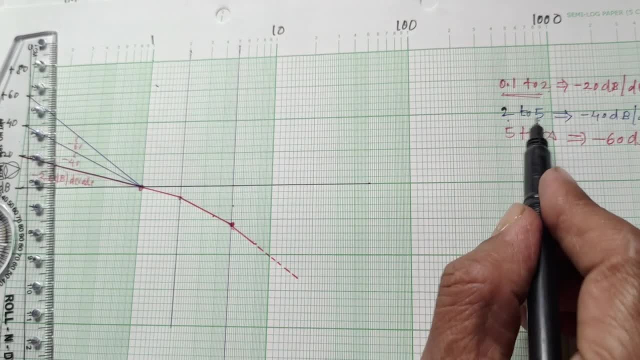 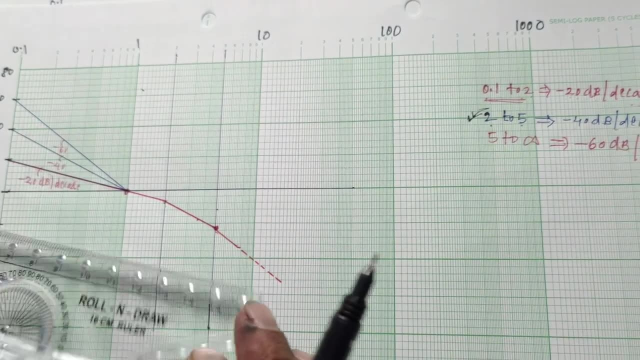 1 and 10. we have drawn a reference line of 2. we have to draw it till 2.5. i am talking about this reading. so this line of 5 is also drawn 2 to 5. now how to draw this line 2 to. 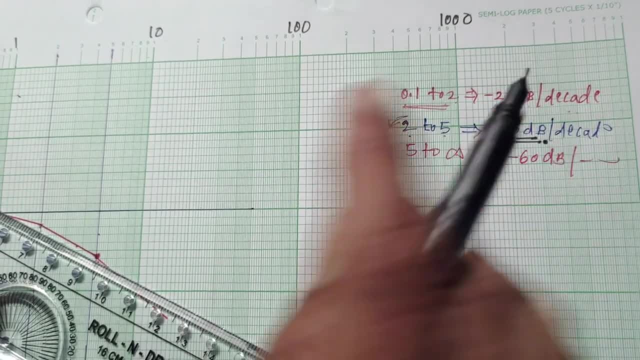 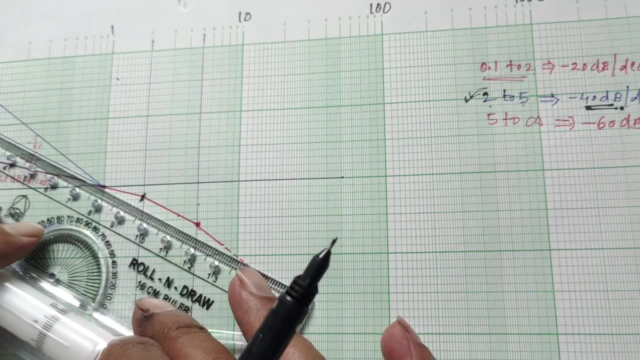 So I need to mark a line whose slope is minus 40 dB per decade. We had done this till 2 earlier. Now see, this is a 40 dB line. We have to use roll and draw to draw it till here. 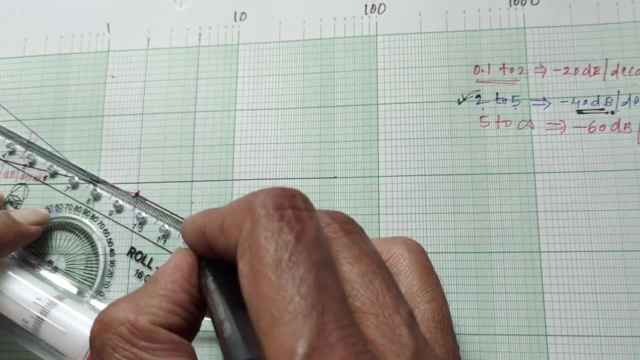 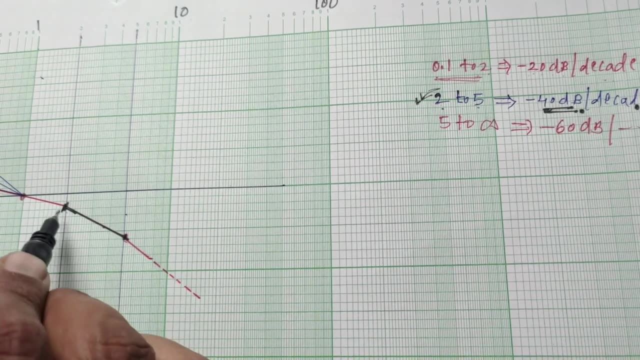 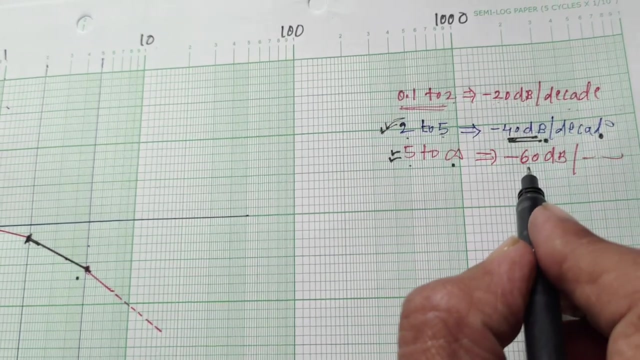 And this line parallel to 40 dB. this line will be having the slope minus 40 dB per decade. I had already drawn this earlier. I have just highlighted it now. Now, last reading, Suppose from 5 to infinity, I need to draw a line of minus 60 dB per decade. 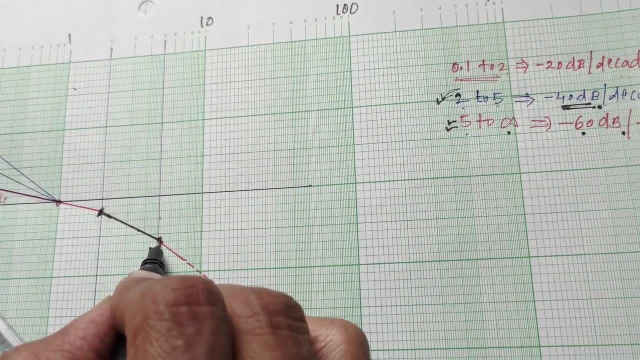 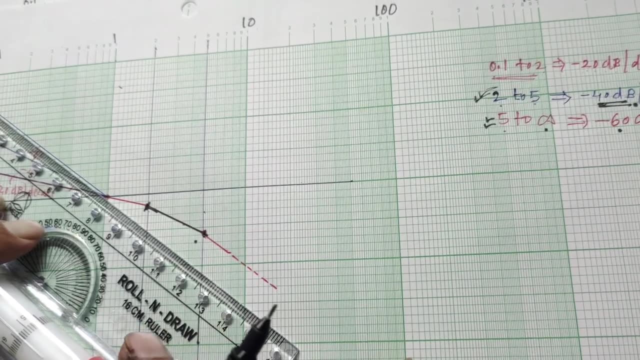 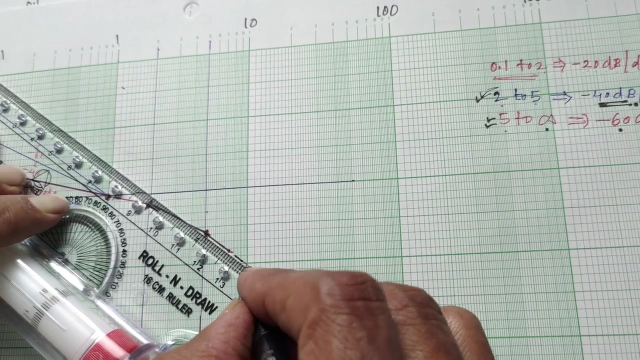 How do I draw this From 5 to minus 60 dB per decade? Refer to this line: minus 60 dB per decade. I will use roll and draw to draw this line from here to infinity. I can't draw the diagram till infinity. 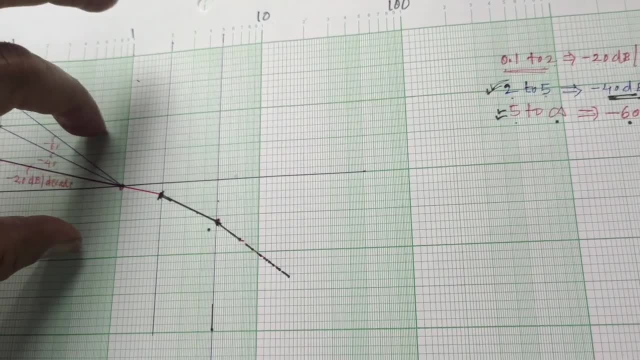 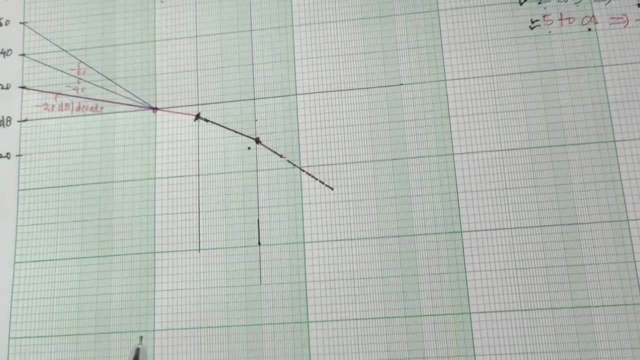 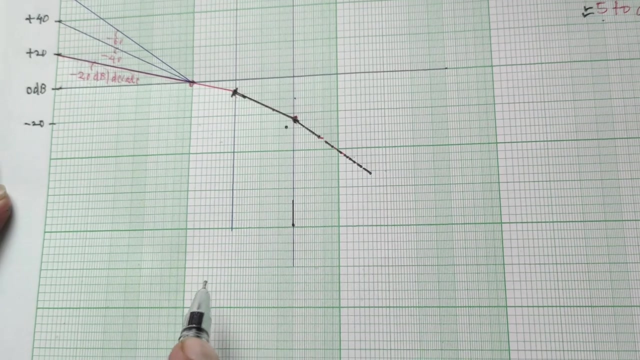 So just mark the dotted line. This is how You can draw the magnitude plot. Now, as I have told you earlier, this is the magnitude plot. Now I have plotted the resultant graph. On that graph paper we need to plot the phase response. 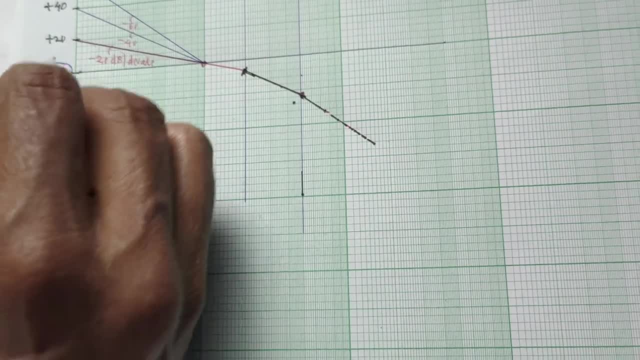 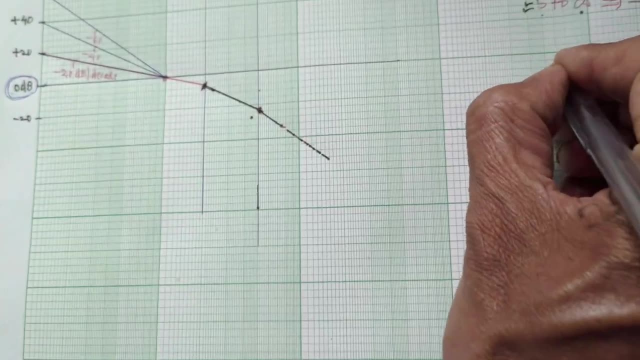 For phase response for magnitude plot you need to take 0 dB as a reference line. For phase plot take minus 180 degree as a reference line. So I will mark here: Minus 180 degree should be Reference point for phasor diagram. 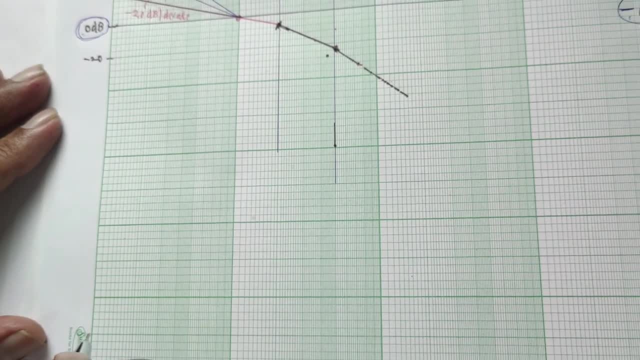 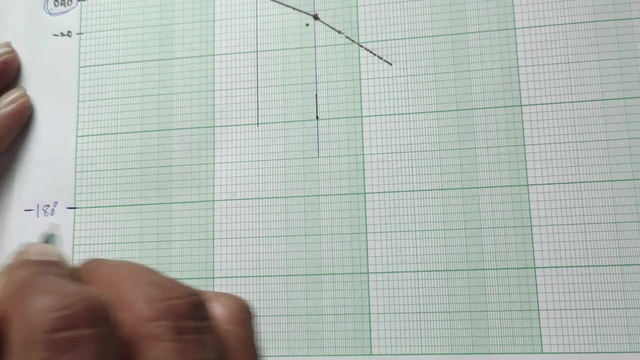 Now somewhere you have to take a little judgment and mark it. Suppose here I assume that this line is of minus 180 degree. Means this line, I am talking about this line, This line. This is corresponding to minus 180 degree. 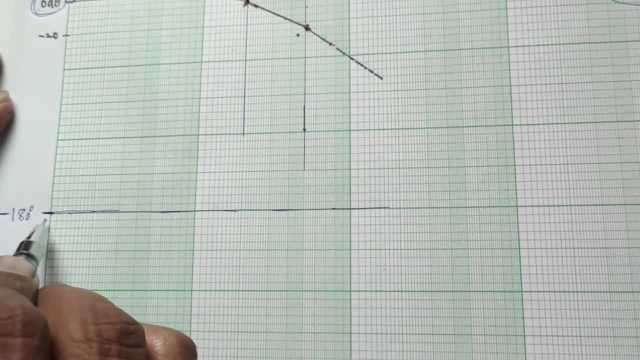 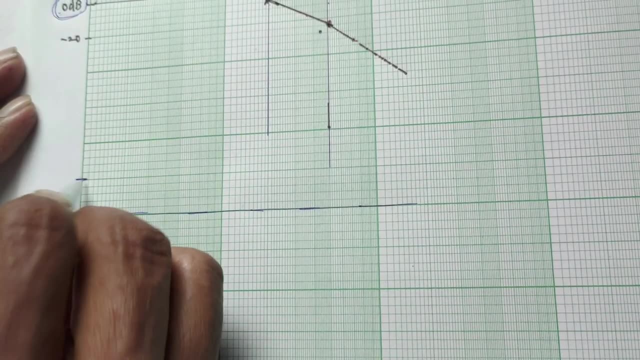 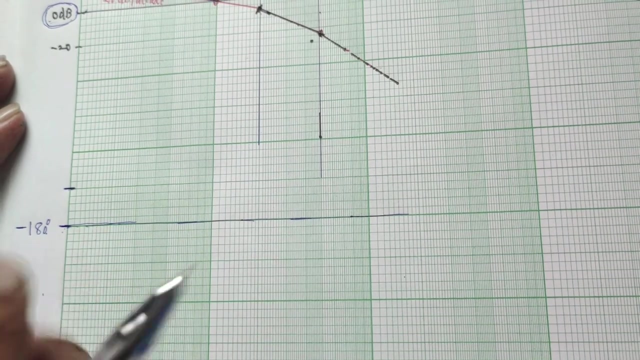 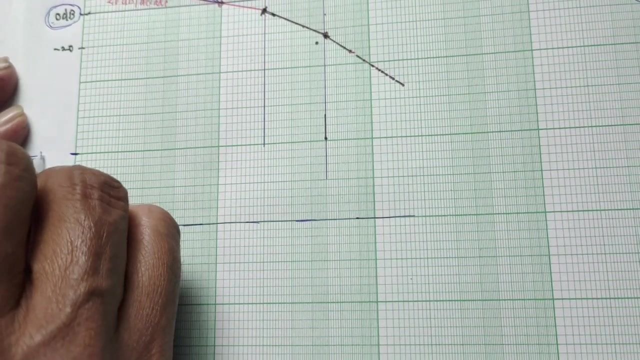 Now listen carefully. Here there is no plus, minus reading. Every reading of phase is negative, So it is minus 180. Next. Similarly, the next slot is of minus 120 degree. I assume that this is a 30 degree slot. 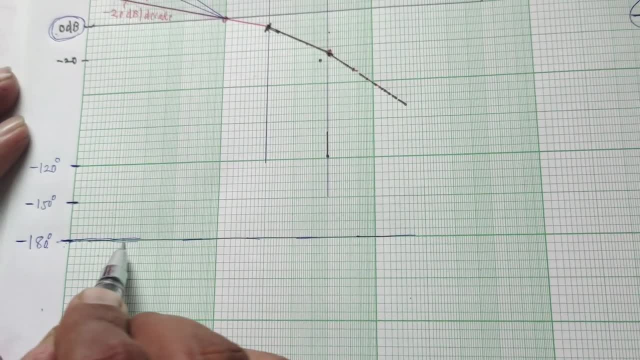 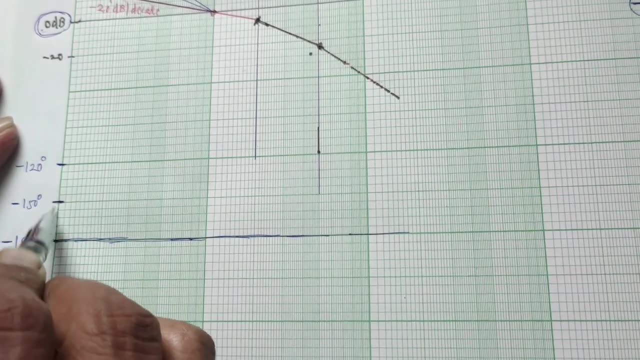 The other slot is 30 degree slot. This is a clear cut assumption. You can well change the reading, So it is a reading of minus 150.. Likewise, I am assuming that this is slot of 30 degree, so this is of minus 150..